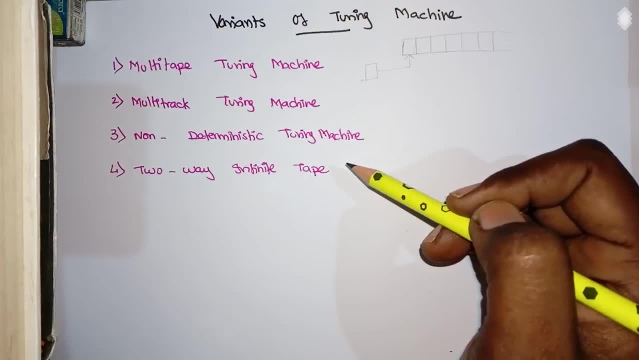 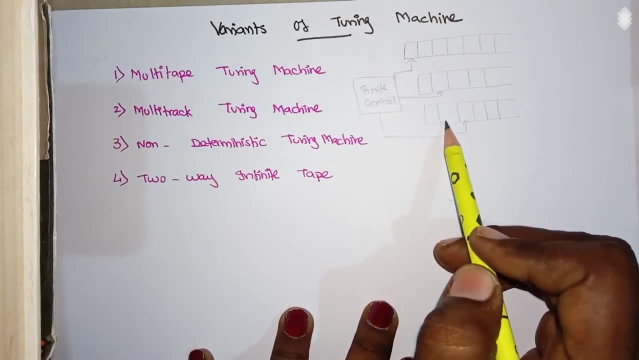 So these are all different ways in which we can simulate a Turing machine. Ok, we will see one by one now. First one is a multi tape Turing machine where you have multiple tapes, So each are all infinite multiple tapes, and we have a single, finite control And as per. 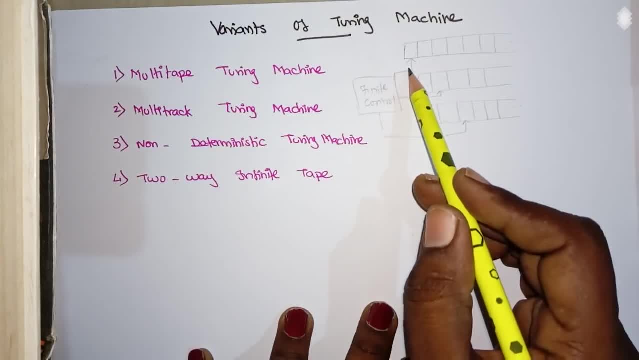 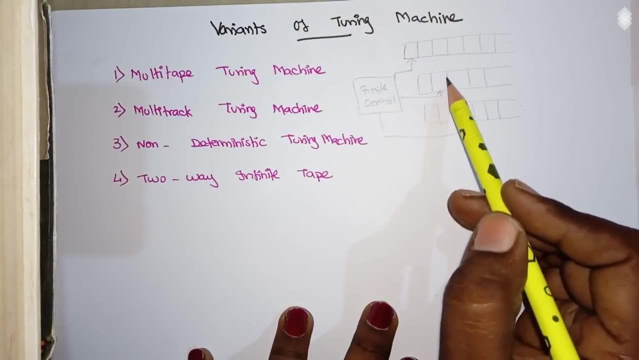 the number of tapes we have. number of read write head: Ok, so each can read at a single time of transition. This read write head can read this tape and this can read this tape read this tape and this can't read this tape. so the transition varies according to the tape number. 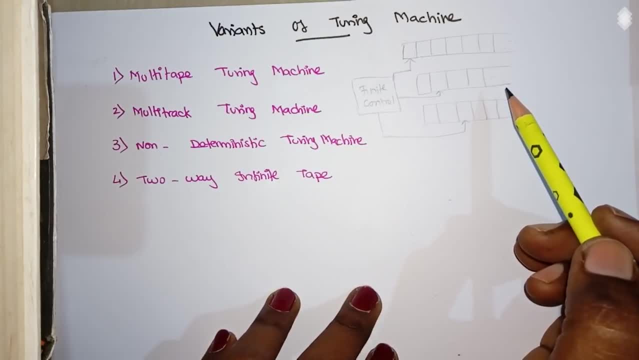 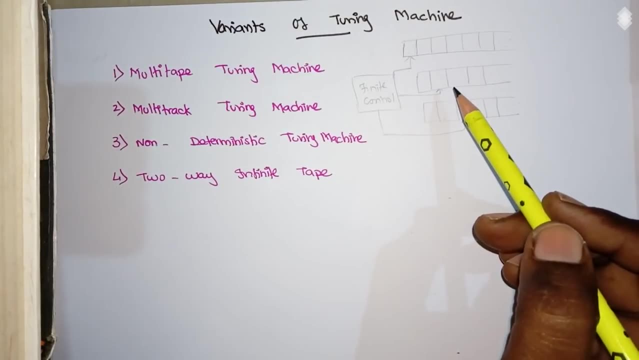 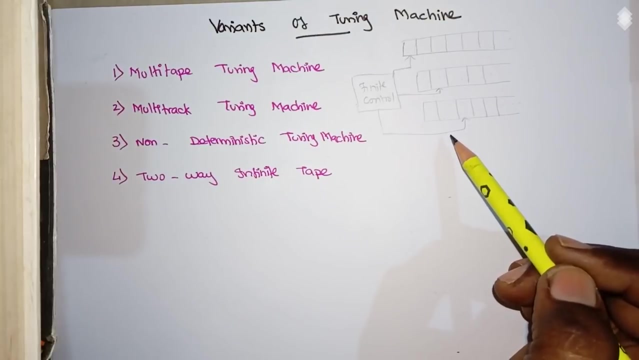 two, okay so, and in the transition we have to mention which which stay or in which tape you are going to make the transition. okay, that is multi-tap turing machine. uh, multiple tapes and with the multiple read write head, with a single finite control. okay, and next one is multi-track. 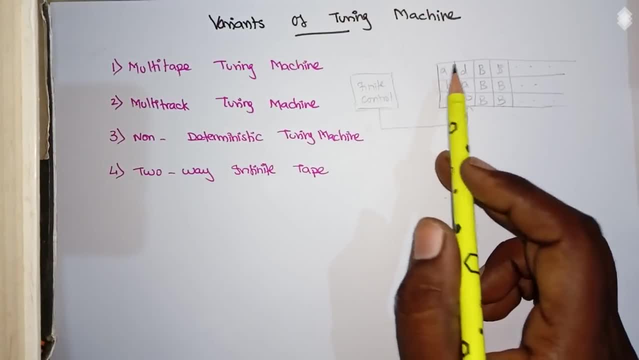 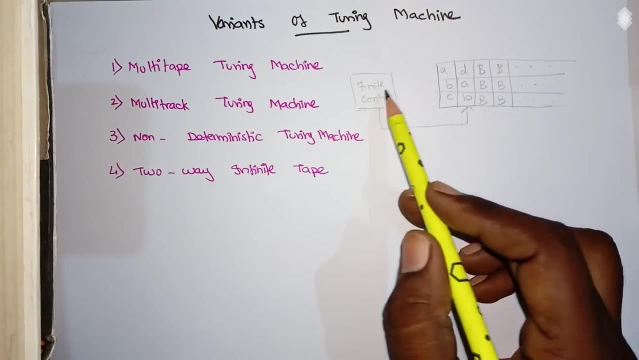 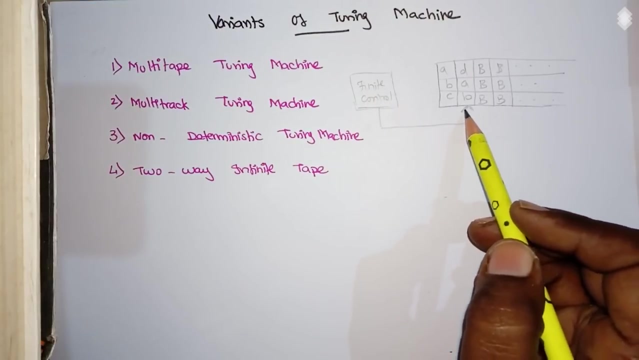 turing machine here, instead of a single track in a single tape. instead of a single track, we can have a multiple tracks at a time, whereas we can have only one finite control. and here also we just have a single read write head. but this read write head is capable of reading all the tracks. 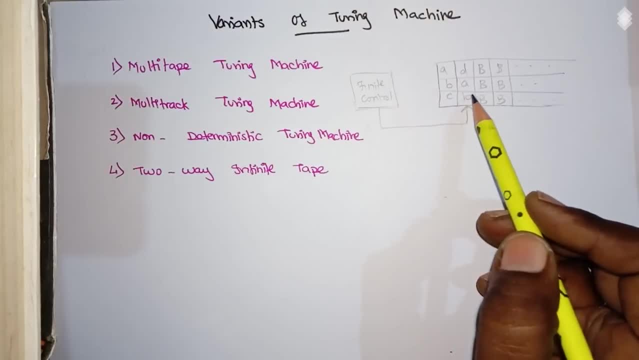 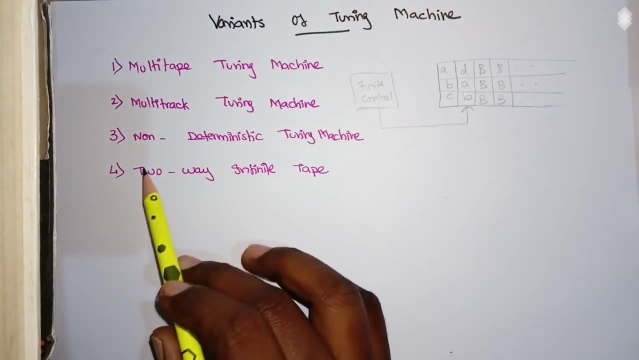 at a time, so the transition is based on all the inputs at a single time. okay, so this is multi-track turing machine. another variation: you can make it in a turing machine, and next one is a non-deterministic turing machine and non-deterministic turing machine. 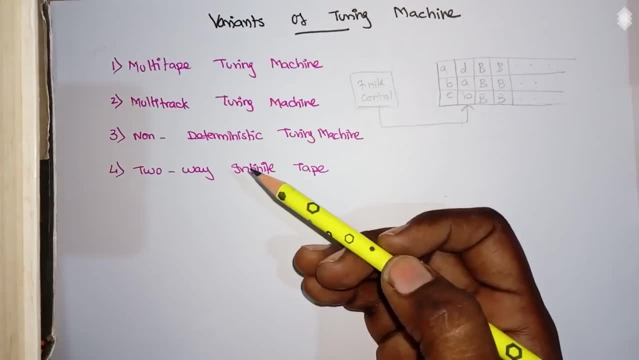 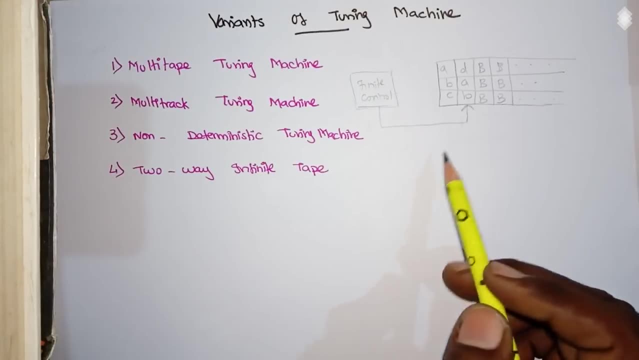 is similar to the top and non-deterministic finite automata or non-deterministic pushdown automata. okay, so while solving some problems, we have to compute parallelly. okay, we'll have some n number of branches at a time. if any one branch goes to accepting we, we have to accept it, okay. 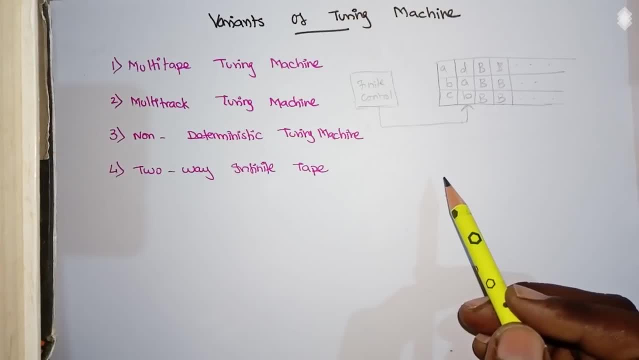 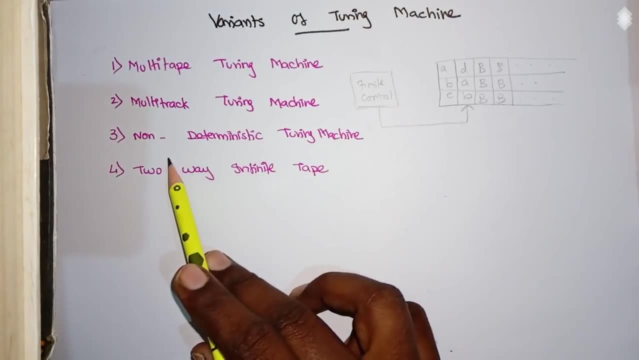 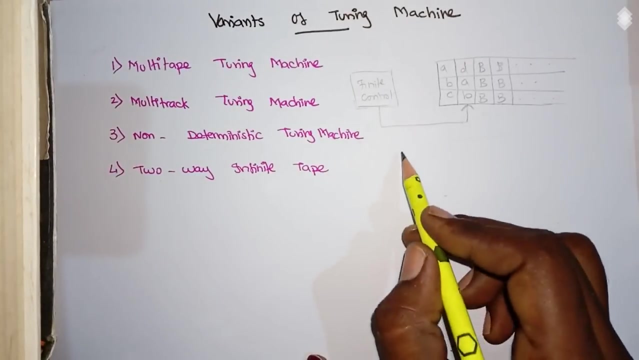 for a single step of transition. you have. you may have. instead of having a single solution, you may have different possibilities too, so that is also allowed in case of a turing machine. so that will be your non-deterministic turing machine, and the last one is two-way infinity. see, here, till now, we have a turing machine and we always assume, 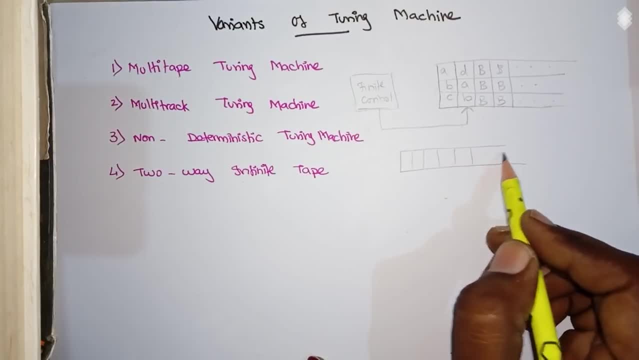 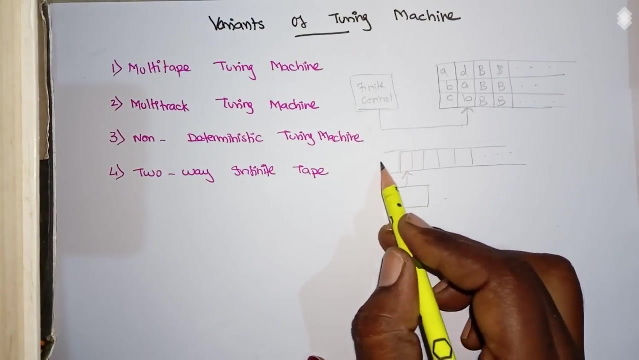 that this tape of a turing machine is freezed at the place. okay, in this end the tape is freezed. okay, and it is infinite in one way alone. okay, so we can have a turing machine that is infinite in two ways too. okay, so that is called a two-way infinite tape. so these are all the. 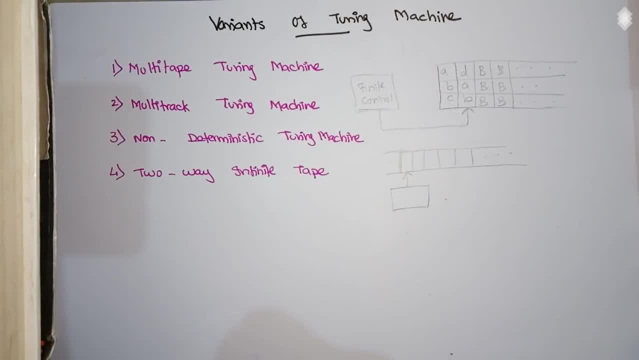 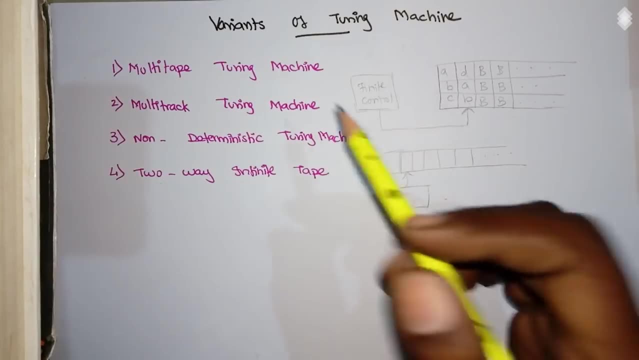 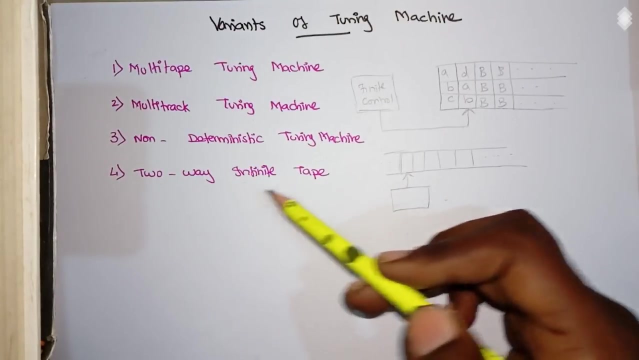 different ways in which you can express a turing machine. even though we have a different ways in different variations in a turing machine, it is all equivalent in the sense, like a multi-day turing machine or a multi-track turing machine, or a non-deterministic turing machine or a two-way. 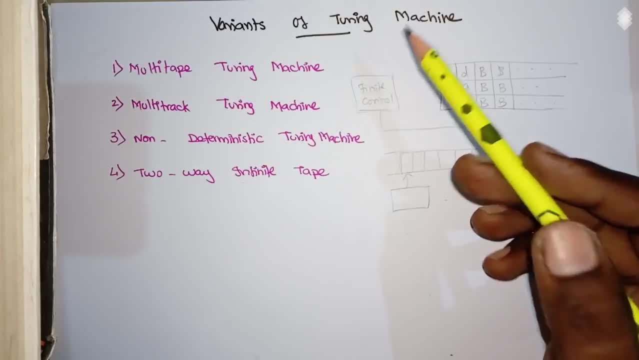 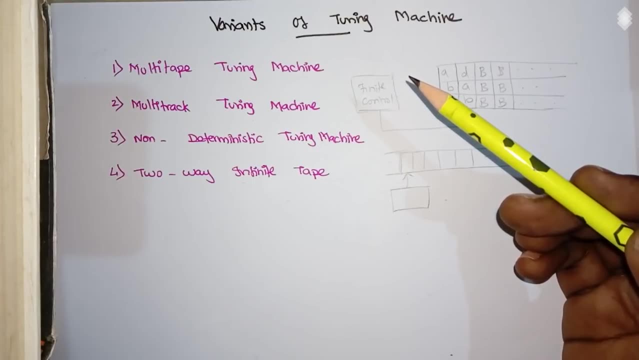 infinite turing machine. it is similar to that of your normal turing machine. it is equivalent to that of a normal turing machine. okay, so how will you prove an equivalence of two machines? see, we have seen that non-deterministic finite automata and deterministic finite automata are equivalent by showing the 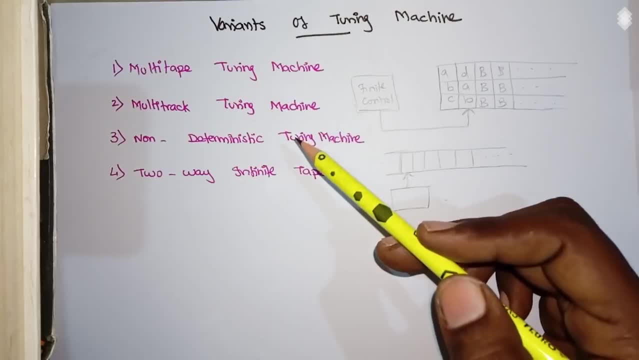 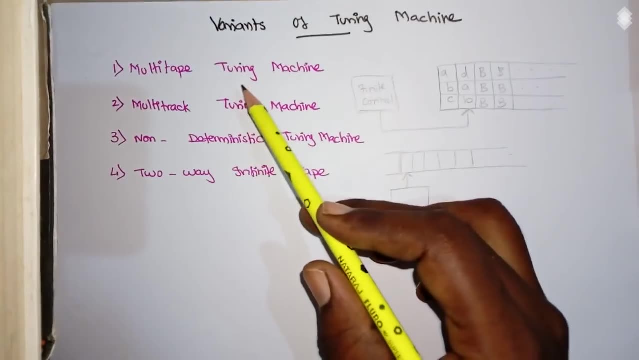 way of conversion. okay, we, we can convert one way machine to other way and the vice versa offered. then we can say that the machines are equivalent. similarly, when you have a way to convert this multi-tap turing machine to a normal turing machine and a normal turing machine to a 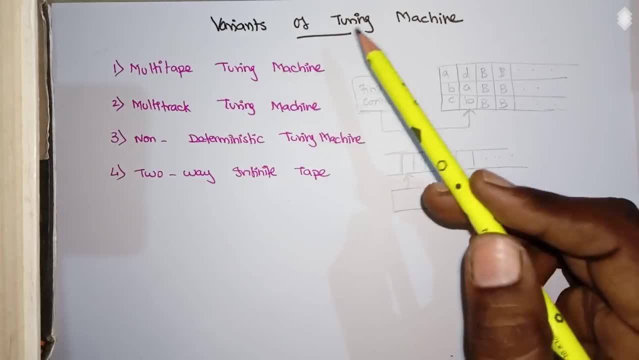 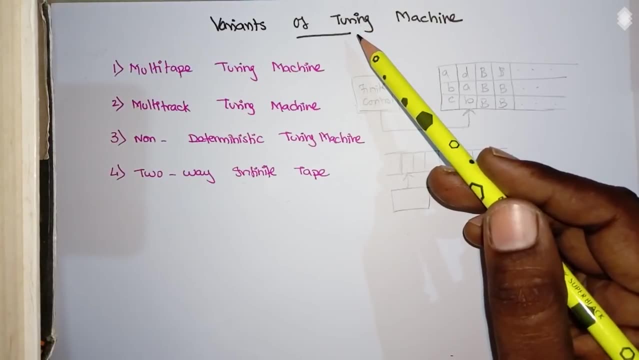 positive turing machine, we can say that that is equivalent. okay, so all these turing machines are equivalent to that of your normal turing machine. okay, so we'll see the proof in the next video. as of now, just know what are the different ways, different variations that exist for a turing. machine.